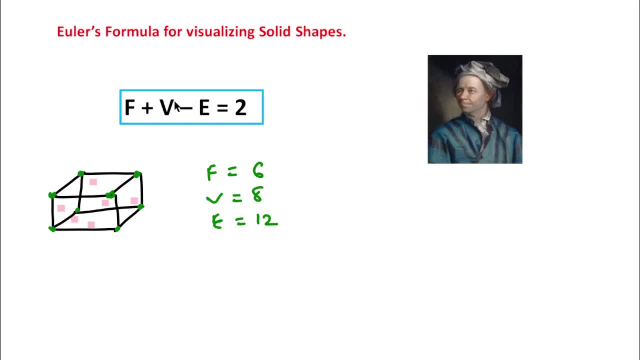 That is, a is equal to also 12.. If you put this value, that is f plus v minus e, means lh is equal to. Then you will get: f is 6 and v is 8 and e is 12.. Then 40 minus 12, that is 2.. 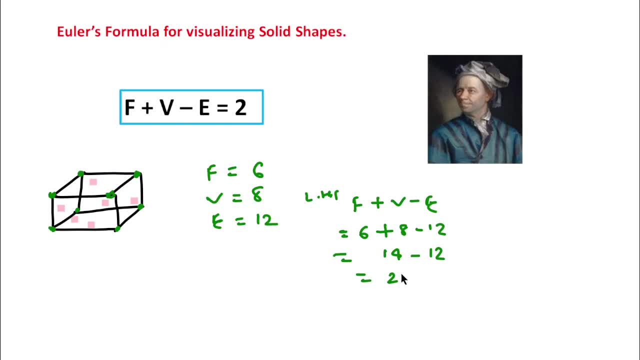 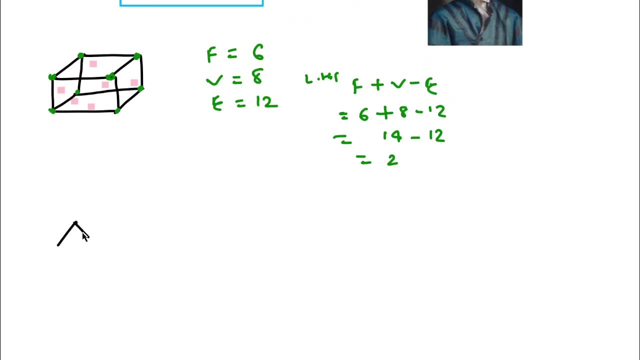 Ok, According to this formula this is true and also for true, For prism also. let's suppose this is a prism, triangular prism. In this prism also, how many faces are there? 1,, 2 and 3,, 4 and bottom. 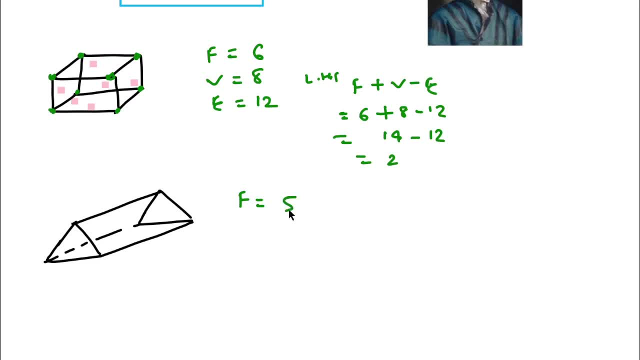 That is 5 faces. and how many vertices? 3 this side and 3 this side. that is 6.. And how many edges? 3 this side and 3 this side. 3 plus 3 is 6 and 3.. 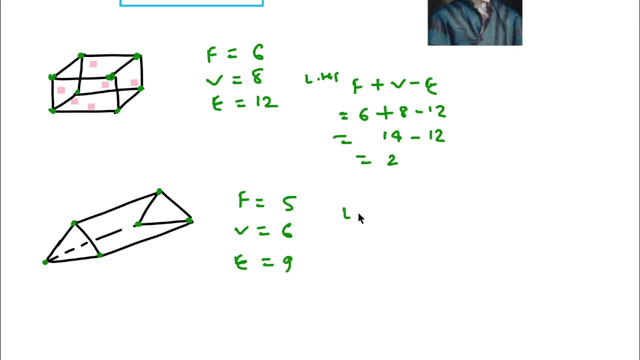 1, 2, 3 also, that is 9.. If you put this value, that is, lh is equal to f plus v minus e, Then you will get 5 plus 6 minus 9.. 11 minus 9, that is also 2.. 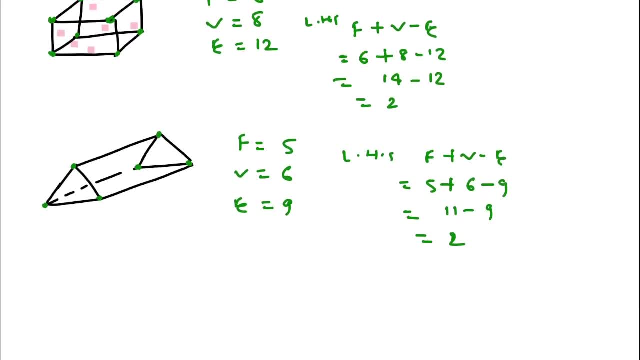 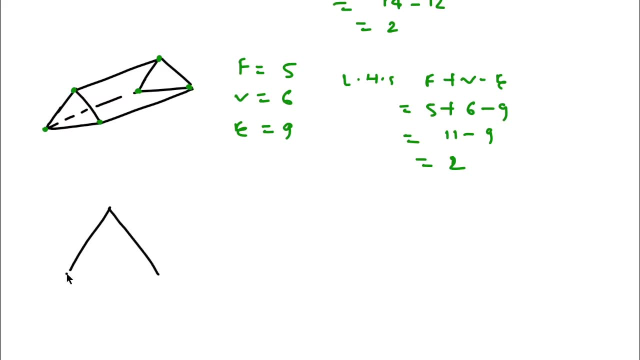 According to formula. this is true, And also for pyramid it is true. Let's suppose this is a pyramid, You notice here. then how many faces are there here? 1st, 2nd and this side also heard total, 3 and 4.. 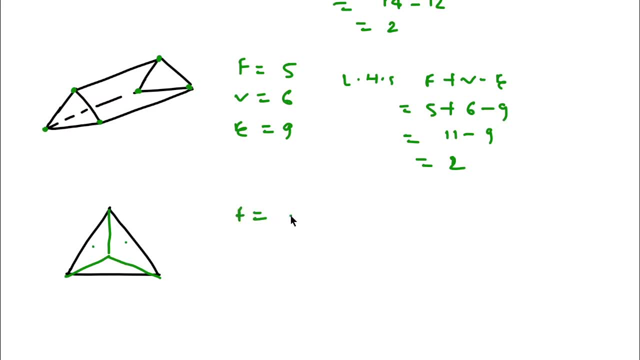 4 faces are there, Okay, And how many vertices: 1,, 2,, 3, 4.. There is a 4 vertices And how many edges: 1, 2,, 3,, 4,, 5, 6.. 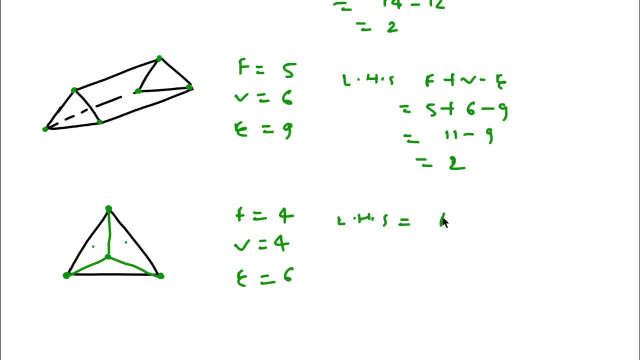 That is total 6.. Then lh is equal to f plus v minus e, That is f is 4 and vertices is also 4. And edge is 6.. Then 8 minus 6.. It is also true for this, Okay.